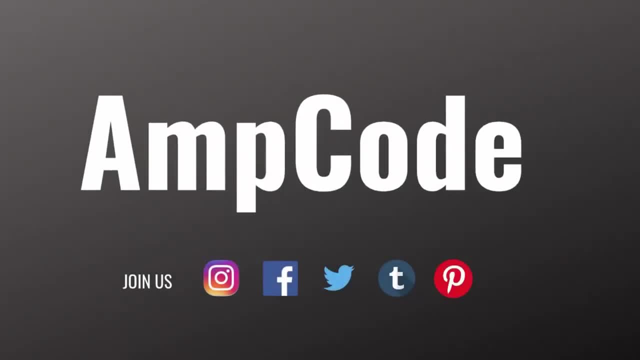 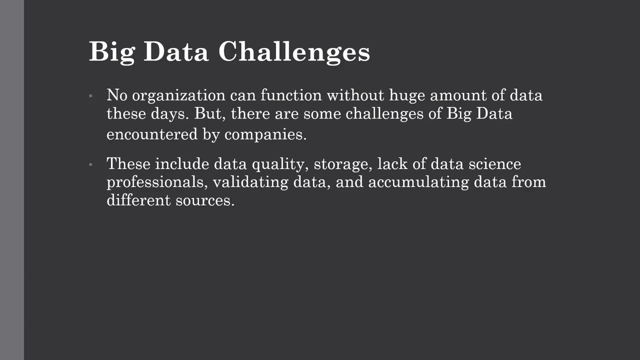 Hello and welcome back to the channel. So in this lecture we are going to talk about some challenges that you might face if you are implementing big data in your organization. So without further ado, let's get into it. So nowadays, no organization can function without 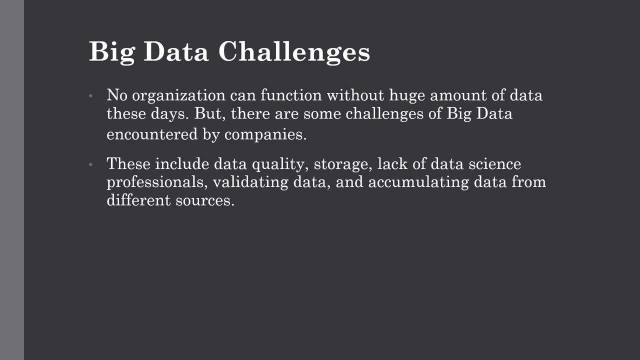 a huge amount of data these days, So big data challenges includes the best way of handling the numerous amount of data, which will involve the process of storing then analyzing a huge set of information on various data source. So there are major challenges that come into 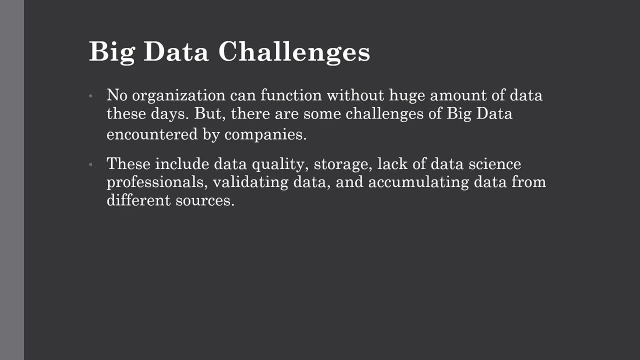 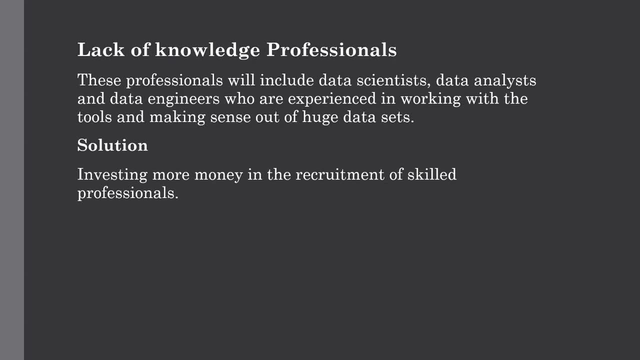 way when we are dealing with big data which needs to be taken care of. And now we are going to see each challenge one by one and how we can resolve them. So the first challenge is lack of knowledge professionals. So to run these modern technologies and a larger 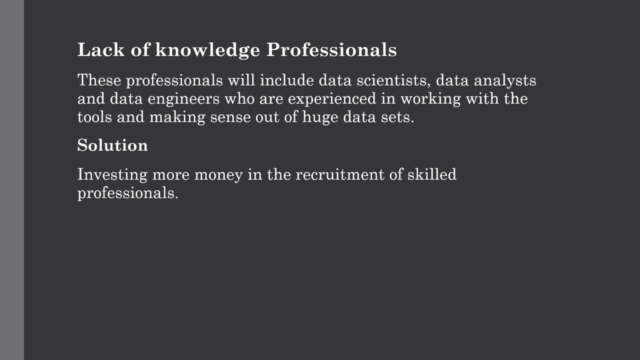 data sets. Companies need a skilled data professionals, So this will include data scientists, data analysts and data engineers- to work with the tools and make sense of a giant data set. So one of the big data challenges that any company might face is a lack of massive data. 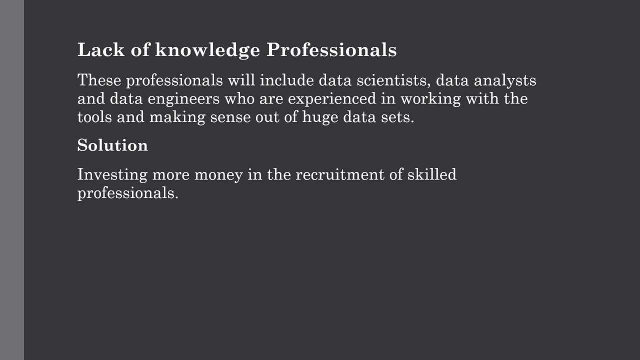 professionals. So this is often because of the data handling tools, which have rapidly evolved, But in most cases the professional haven't. So now we will see what are the actionable steps that we need to take care to bridge this gap. So the main solution being here is: the companies has to invest extra money in recruitment of 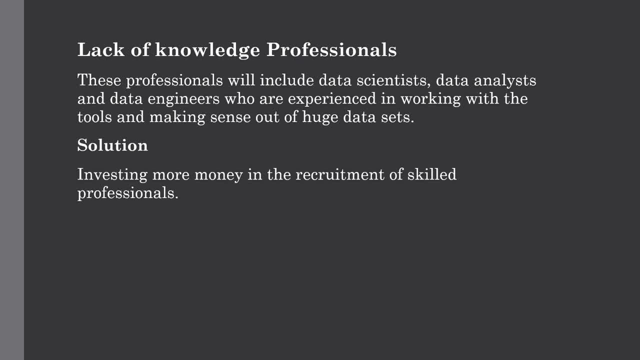 skilled professionals, And they even have to supply training programs to the prevailing staff to usher foremost out of them. Another important step taken by organization is purchasing knowledge analytics solution, which is powered by AI and ML, So these big data tools are often traveled by professionals. 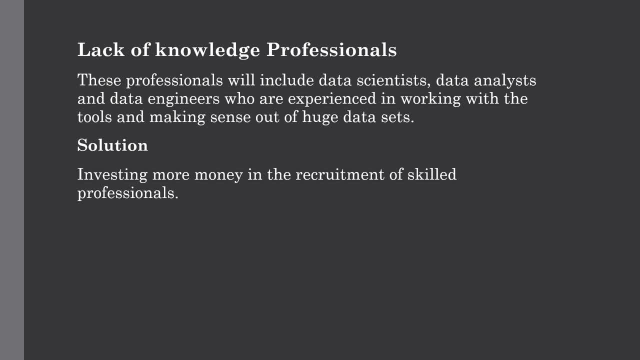 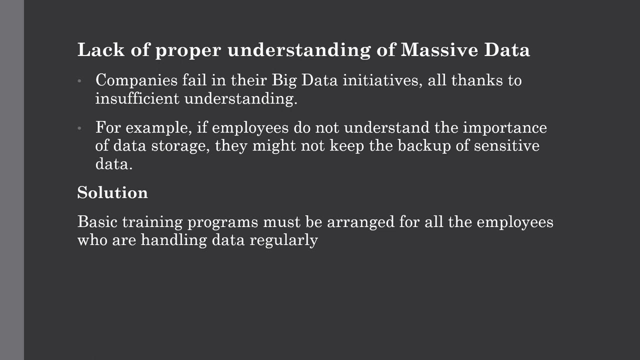 So this step will help companies to save a lot of cash for the recruitment. The second challenge is the lack of proper understanding of how massive the data is, So the companies fail in their big data initiatives. all thanks to the insufficient understanding. So employees might not know what data is, its storage, processing importance and the 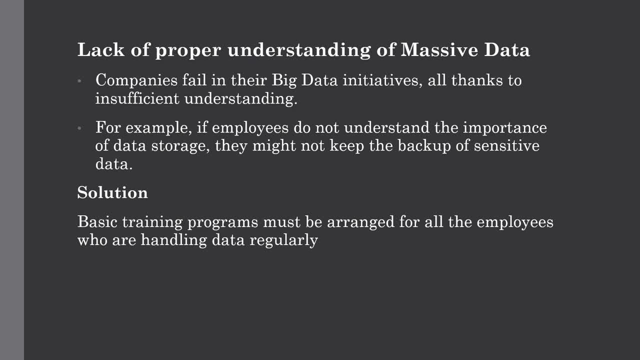 different sources, So data professionals may know what's happening, but the others might not have a transparent picture. For example, if employees don't understand the importance of knowledge storage, they could not keep the backup of sensitive data And they could not use databases properly. 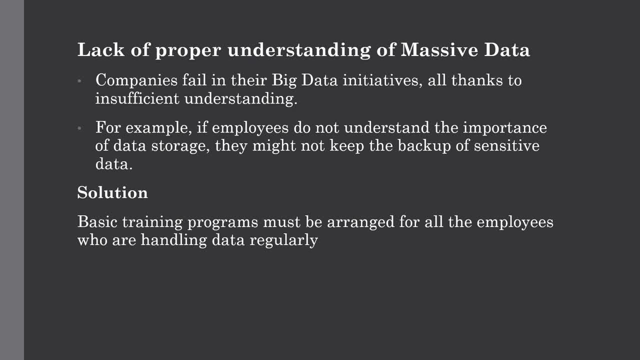 for storage. As a result, when this important data is required, it can't be retrieved easily. So we can overcome this by the big data workshop and seminars. So we can overcome this by the big data workshop and seminars. So we can overcome this by the big data workshop and seminars. 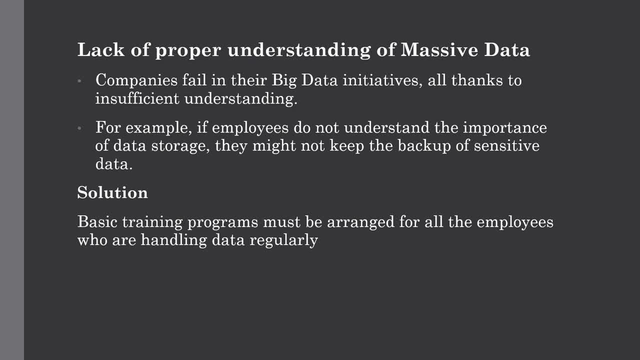 This is the challenge which we must face. The challenge is for company to recover the data that they use to Odinく manage the data, what I am using now, So a big data workshop, is a good idea for the company to deliver. using this someday, I would like to generate 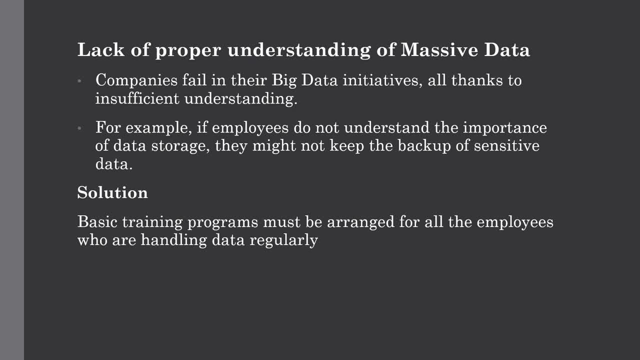 Big data workshops and seminars. Then, for the bigger data workshop to work and deliver- and I am using large data also For the big data workshop- we have to make the high-quality Clay strawberries. These are the things we need to do in order to get the έχει. they have converted. 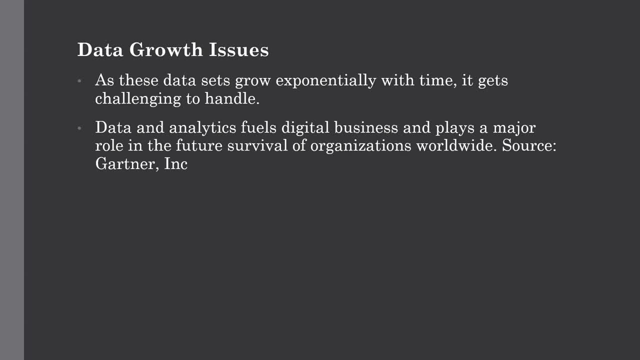 And this has been done before. polygon at the top, massive data, is storing this huge set of knowledge properly, so the quantity of data being stored in a data center and databases of companies is increasing at a huge amount. so as these data cells grows exponentially with time, it gets. 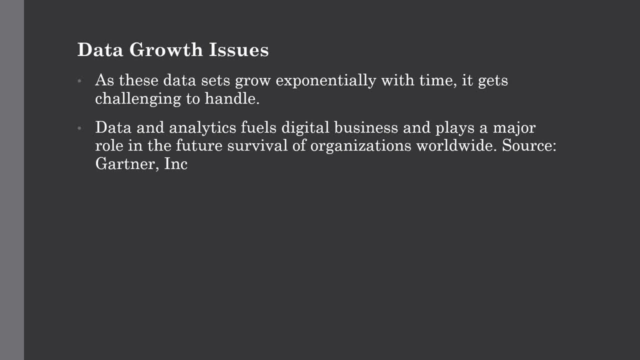 challenging to handle and most of the info is unstructured and comes from either documents or videos, audios, text files and other sources, so this suggests that you cannot find them in a database. so companies choose modern techniques to handle this large data set, like compression, tiering and. 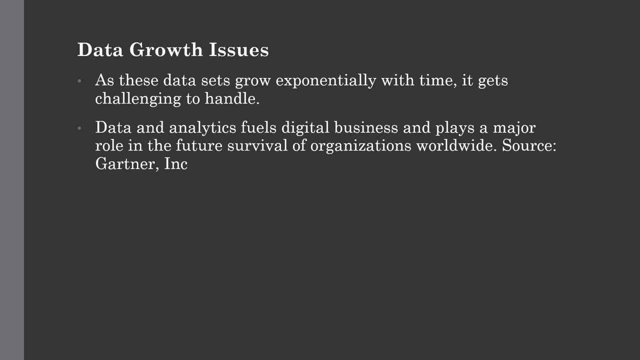 deduplication. so this compression is employed for reducing the number of bits within the data, thus reducing its overall size. and the deduplication is the process of removing the duplicate and unwanted data from a knowledge set. so this data tiering allows companies to store data. 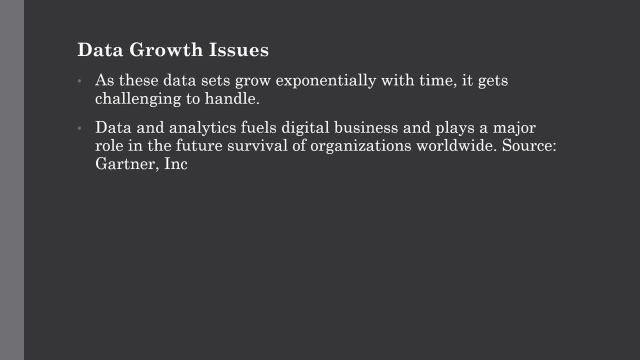 instead of storing it in the database. so this is a very important step in the several storage tiers. So this will ensure that the info is residing within the most appropriate space of storing. So companies are also choosing big data tools like Hadoop, NoSQL and other technologies. 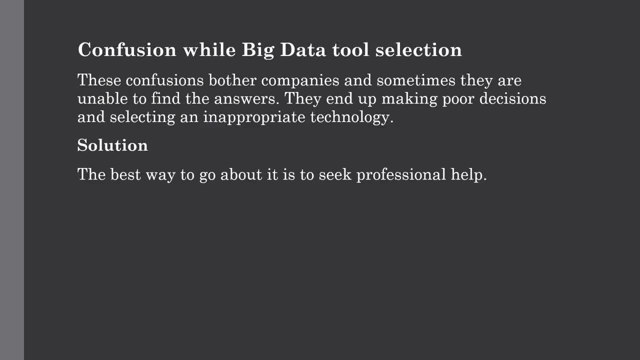 to encounter this issue. So the next challenge is- and it's really important to understand- which is confusion while selecting a proper big data tool. So companies often get confused while selecting the simplest tool for giant data analysis and storage. So you might ask questions like: we should use HBase or Cassandra for simple data storage? 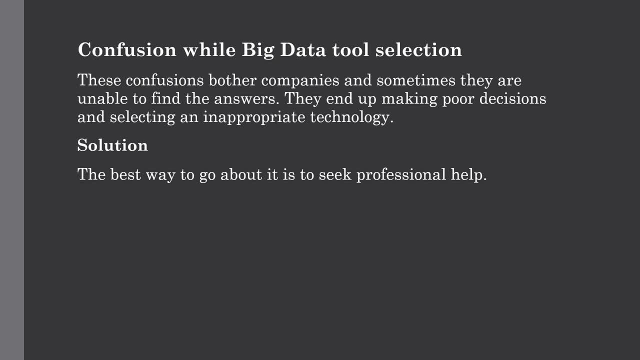 as well, as is Hadoop, MapReduce okay or Sparx be far better option for data analytics and storage? So this question will bother companies and sometimes they are unable to seek out the answer and they find themselves making poor decision and selecting the improper technology. 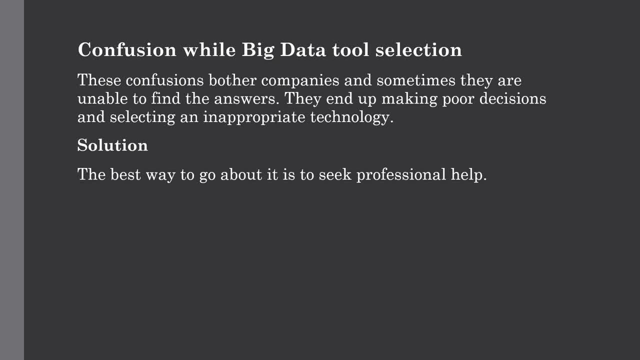 As a result, money, time and efforts are wasted. So how we can tackle this? You will either hire experienced professionals who know far more about these tools. differently is to travel for giant data consulting. So here consultants will provide a recommendation of the simplest tool supporting your company's. 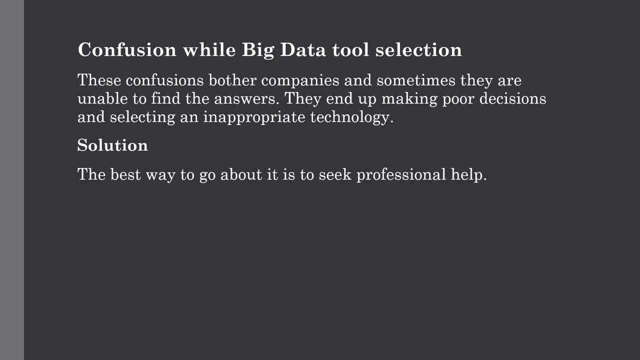 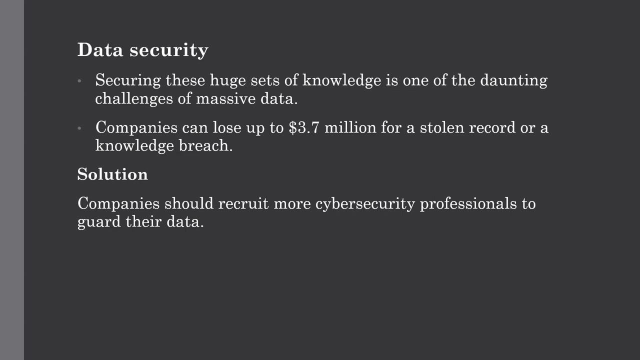 scenario. So it totally depends which type of data your company is consuming, as well as the size of the data set. So, supporting their advice, you will compute a technique, then select the simplest tool for you. So the next challenge is data security. So securing this huge set of knowledge is one of the daunting challenges of massive 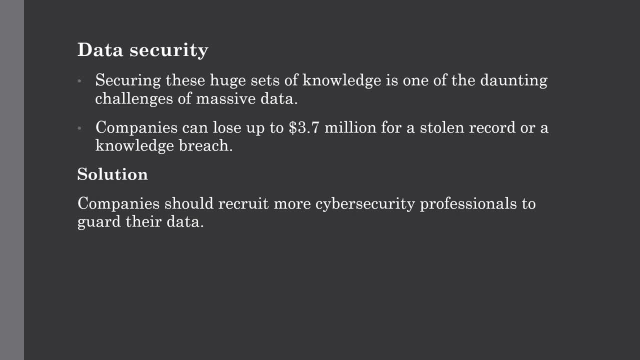 data So often. companies are so busy in understanding, storing, cleaning and analyzing their data that they push data security for later stages. But it is not recommended. This is often not a sensible move, as unprotected data can become breeding grounds for malicious hackers. 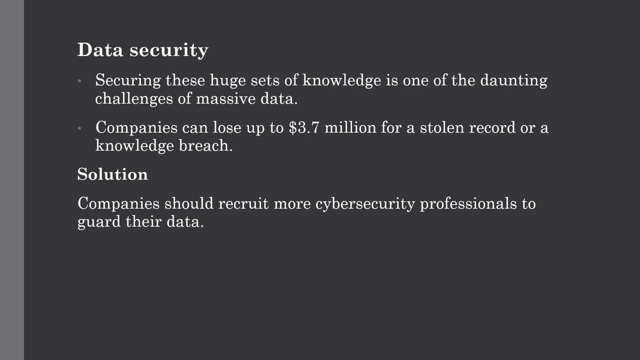 And companies nowadays can lose a lot of data. So the next challenge is data security. So securing this huge set of knowledge is one of the daunting challenges of massive data. So how can we solve this problem? So nowadays, companies are recruiting more cyber security professionals to guard their 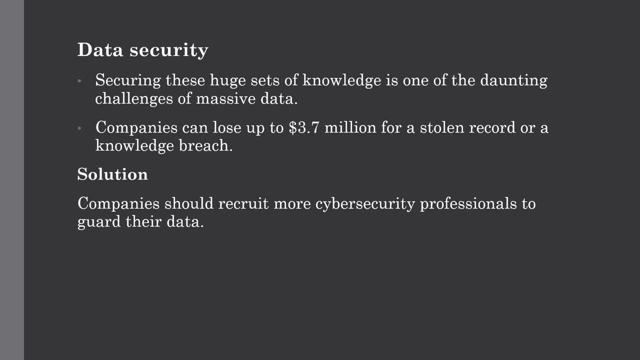 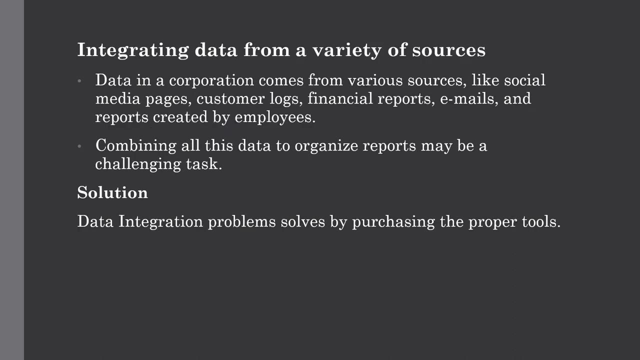 data And as well as other steps for securing big data includes data encryption, data segregation, identity and access control and using the big data security tools like IBM Guardian. So how can we solve this problem, And the last challenge being integrating data from variety of sources.